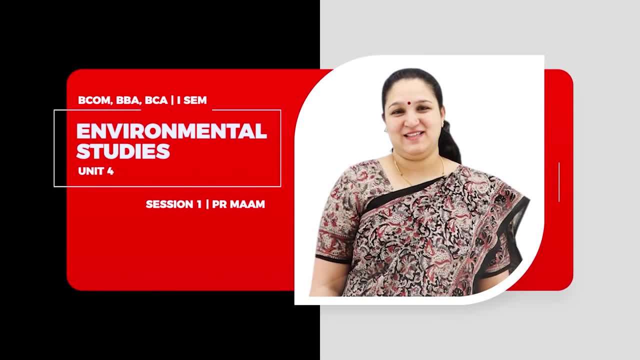 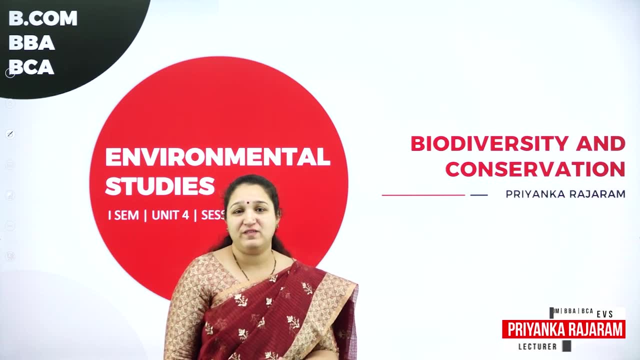 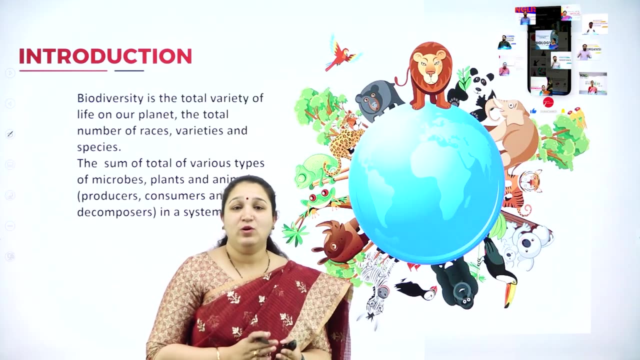 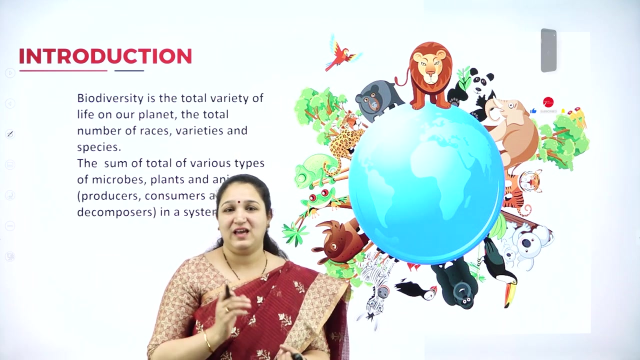 Hello, my dear students. Today I am going to start with the new chapter: Biodiversity and Conservation. So what exactly is the meaning of biodiversity? Biodiversity, the word itself tells. bio means it is the form of life. okay, It can be plants, it can be animals or it can be humans. 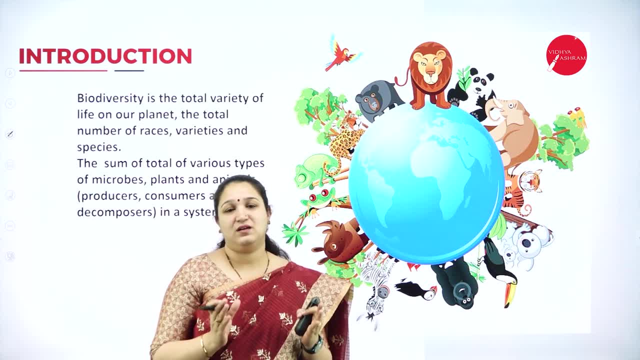 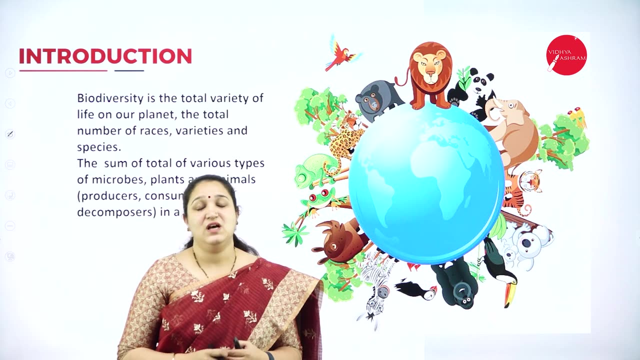 whatever Life means, it is the form of life, okay. It can be plants, it can be animals or it can be humans. whatever is there that is termed as bio diversity means there is different varieties, okay. so biodiversity or biological diversity means the different forms of life or different varieties of life, which is 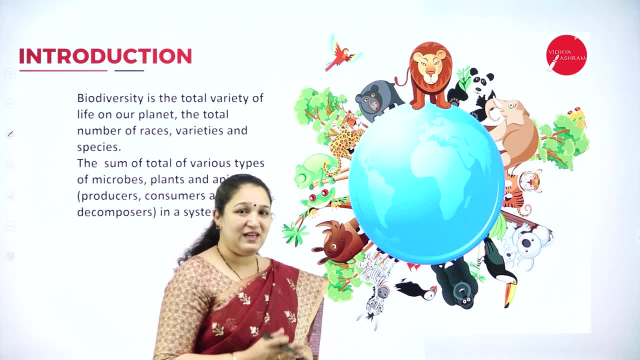 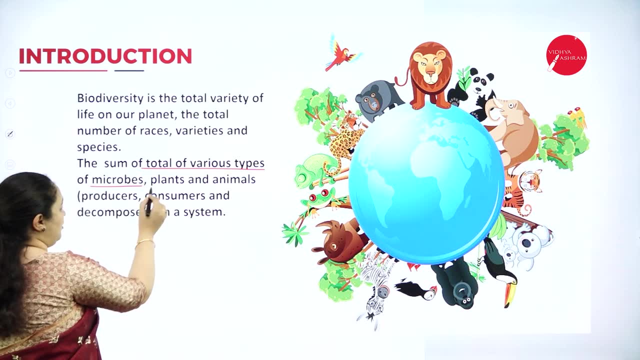 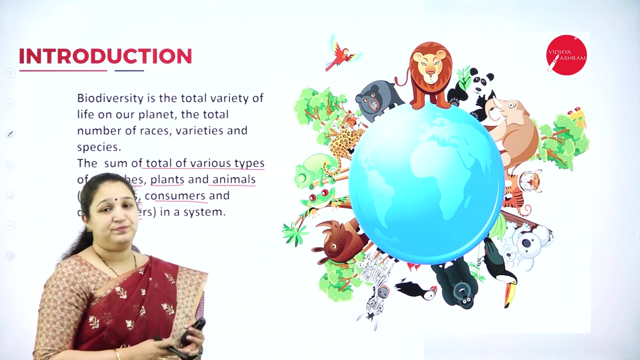 there on earth. so what exactly is the definition of biodiversity? the sum of total various types of microbes, plants, animals, that is, produces, consumers, as well as decomposes in a system, is called as biodiversity. so we are going to learn today about the biodiversity in india, and how are we going to 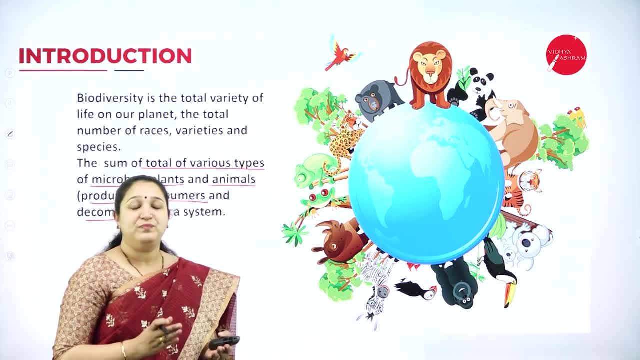 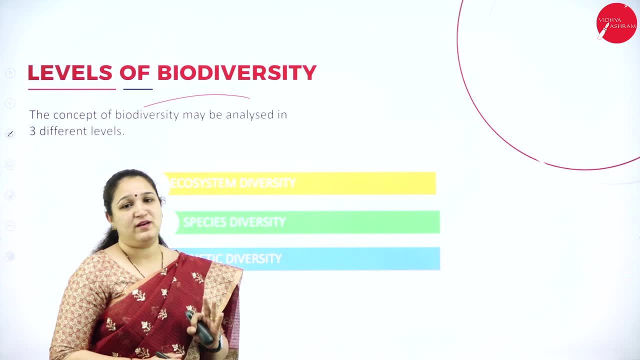 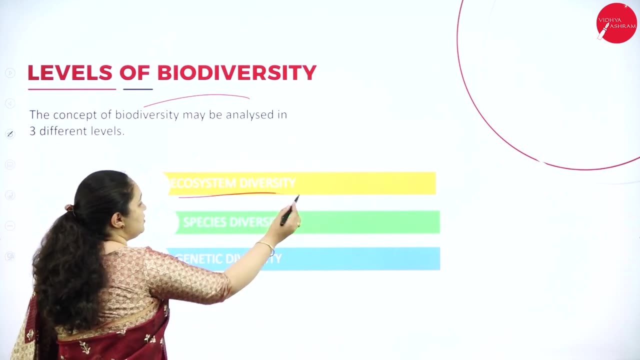 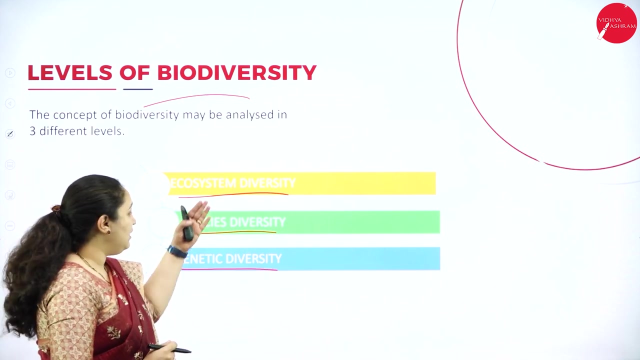 conserve our biodiversity, okay. next we have the levels of biodiversity. there are totally three levels of biodiversity to understand the concept of biodiversity. first one is the ecosystem diversity, then we have the species diversity and then the last one is genetic diversity. we learn each one of them in detail. so first we have 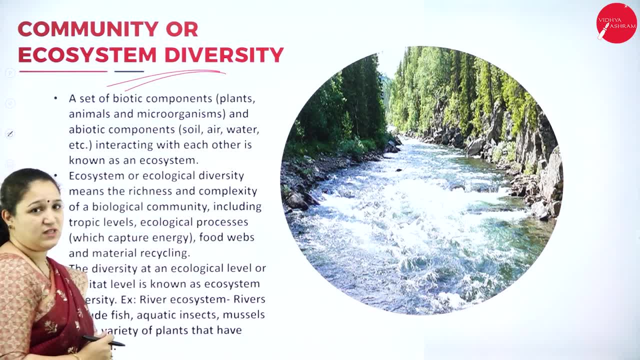 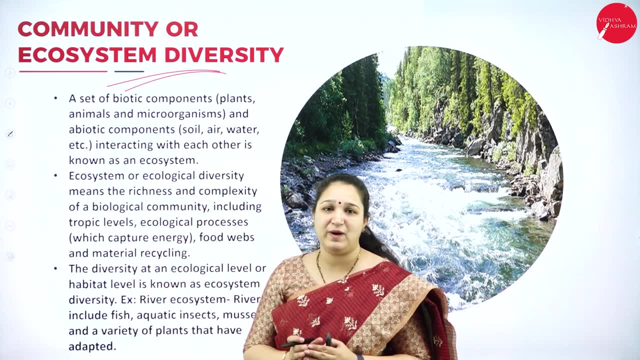 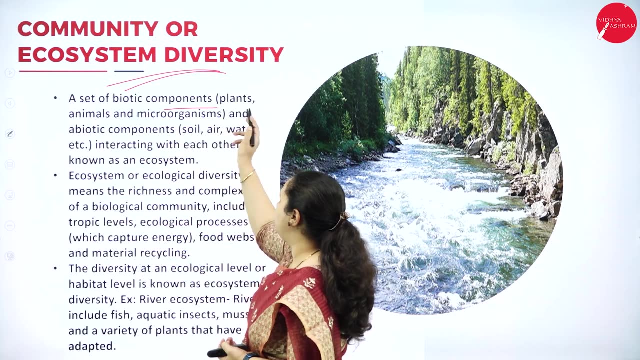 the community or the ecosystem diversity? what is an ecosystem? we have already learned: ecosystem is where the biotic as well as the abiotic components are interacting with one another, isn't it so? we have the biotic components- that is, plants, animals and microorganisms- and the abiotic components. 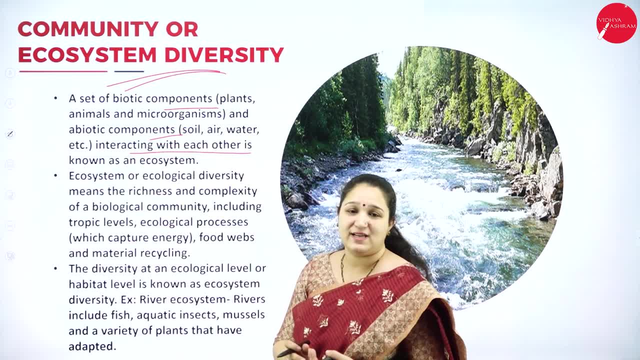 which are interacting with each other is called as ecosystem, and in ecosystem we also learned about the different tropic levels in the ecosystem. so we learned about these. on example, lucian, we learnt about the producers, consumers and then the decomposers as well, and also we have 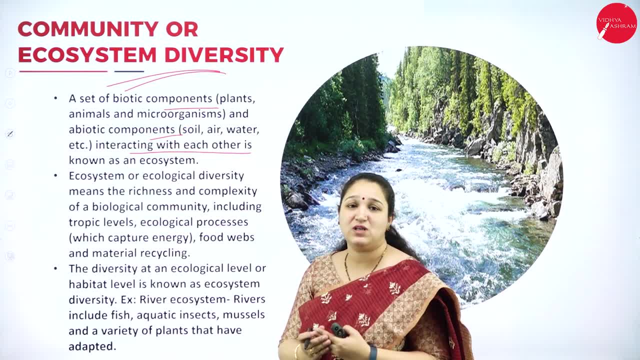 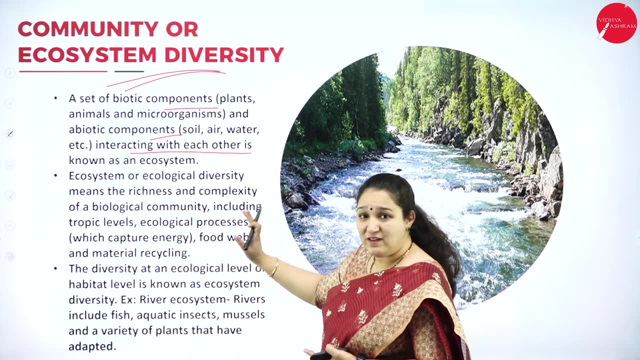 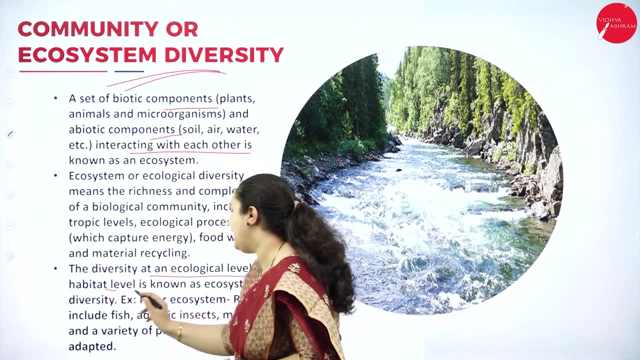 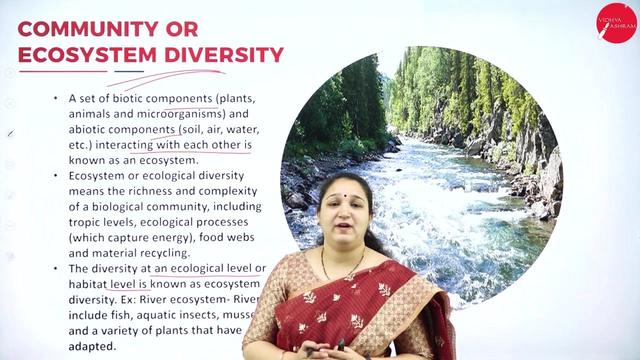 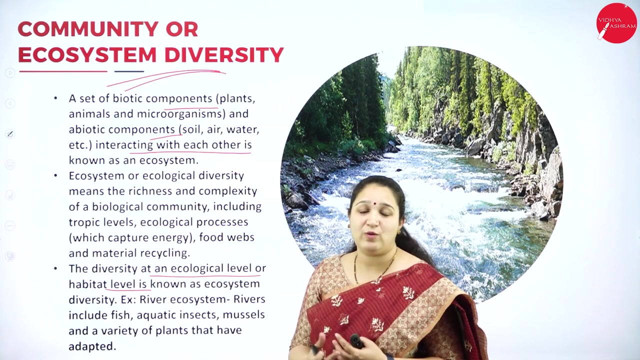 learnt how these are interdependent on one another using food chain and food web concept, isn't it So? ecosystem diversity means the diversity at an ecological level or the habitat level is known as ecosystem or community diversity. For example, if I take river ecosystem, In river ecosystem, what are the different types of aquatic plants which are? 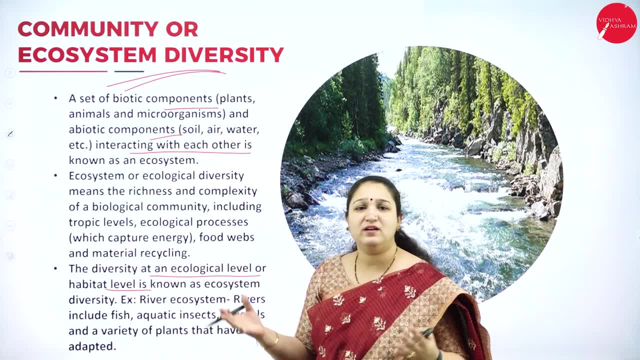 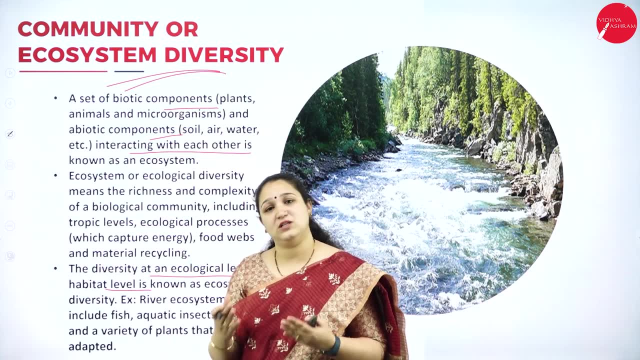 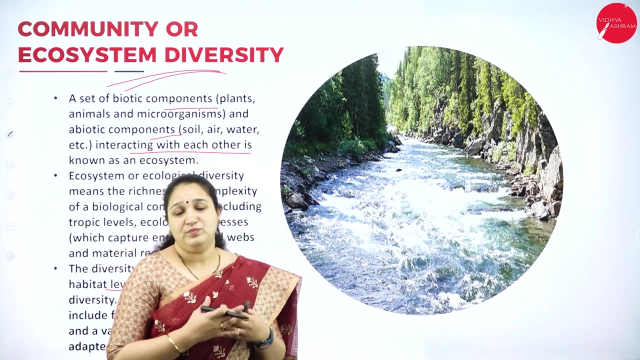 different types of aquatic animals which are there. There is a wide diversity in that That is called as the ecological biodiversity or ecological diversity. There are different types of ecosystem also, which is called ecological biodiversity. There are different types of ecosystem also, which is called ecological diversity. There are different types of ecosystems. 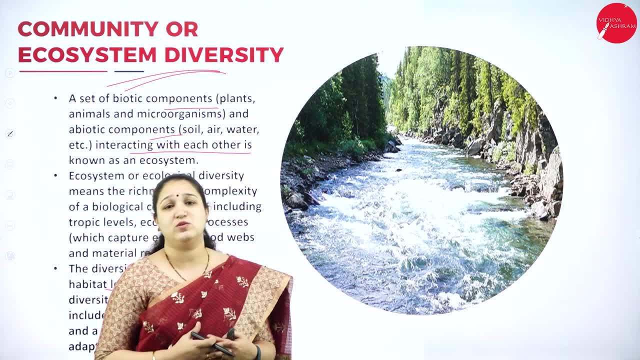 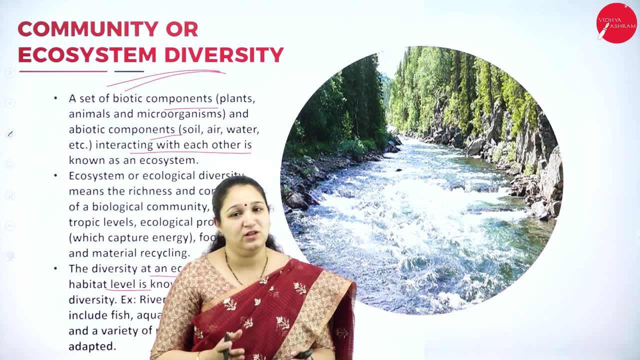 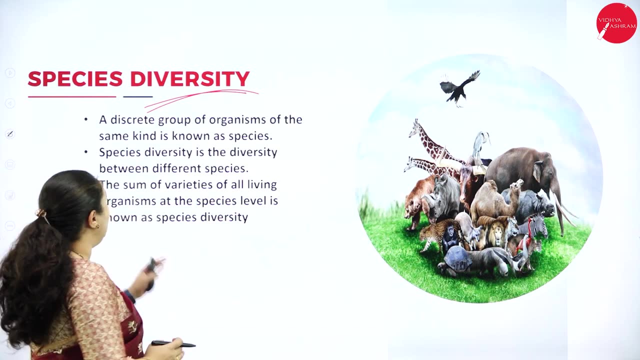 which is called ecological diversity. That is called ecological diversity. That is called ecosystem diversity. That is called ecological diversity. Дod he tree by the Прим rocks, which is very wheat flour, there are a different type of Pten which is than in the earth. that goes into different types. It can be from the forests. to the desert. It can be terrestrial ecosystem, It can be aquatic ecosystem, Different types of ecosystem also. we have studied, which is also under ecological diversity, Species diversity. Now, what is the species diversity? The discrete group of organisms of same kind is known as 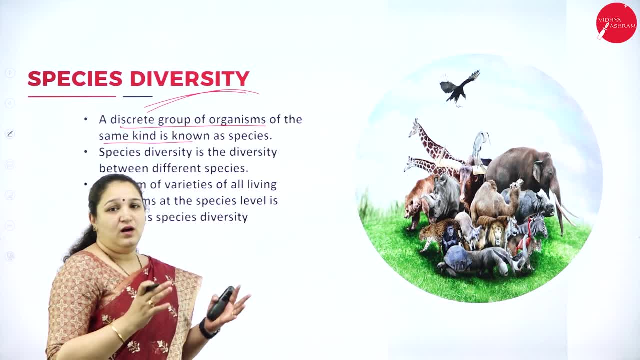 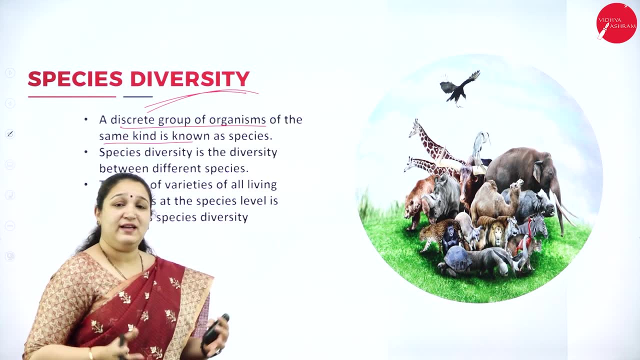 pterignment And even though, because we turn when we carry on using different organisms, shows species. Now, for example, I can take apples. Apple is a fruit, which is a species. There are different varieties of apple which is available. that comes under genetic diversity, So species means it is. 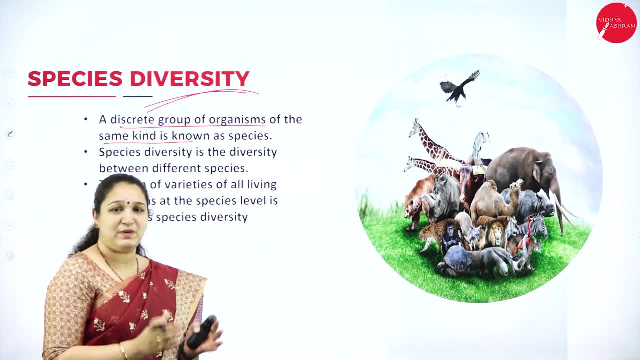 of you know a group of organisms of the same kind, or I can tell you know rice, Rice, we know there are so many different varieties of rice. that comes under genetic diversity, where there is a small change in the gene and you are getting the different varieties, But which is the species? 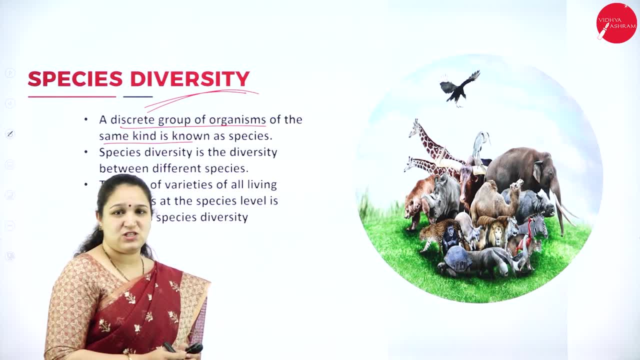 Species. is rice okay or cat species? if you take Cat, is a species, okay, but it has got different. you know life. or it can be tiger to house cat or, you know, to Persian cat. different, different types of cats are there. That is again the genetical variety which is giving rise to 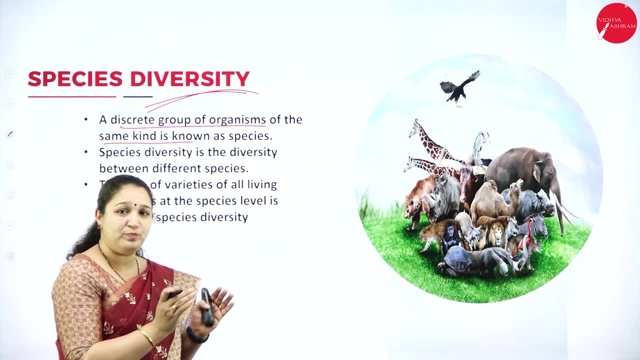 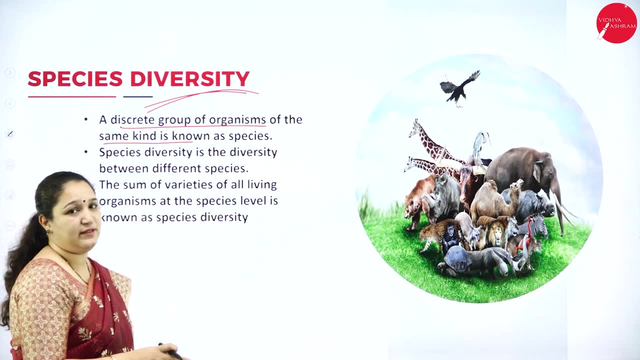 So many different types. but all of this belongs to which group? Cat species. okay, A species is what It is: a group of organisms of the same kind. okay, Species. diversity is the diversity between different species. So how many different species are there? which is living on the earth, That is? 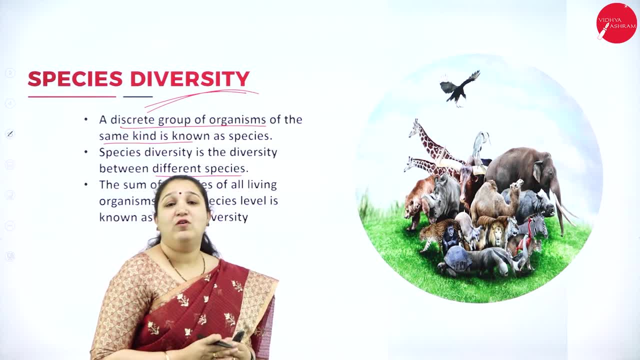 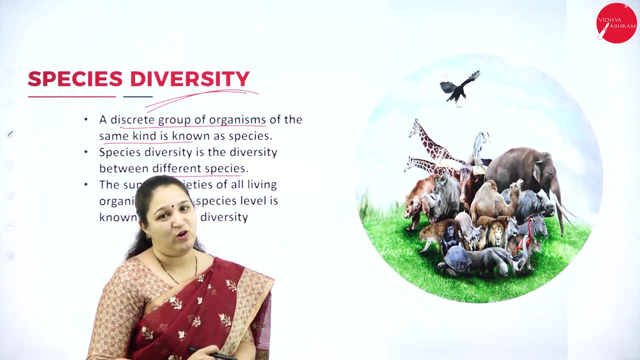 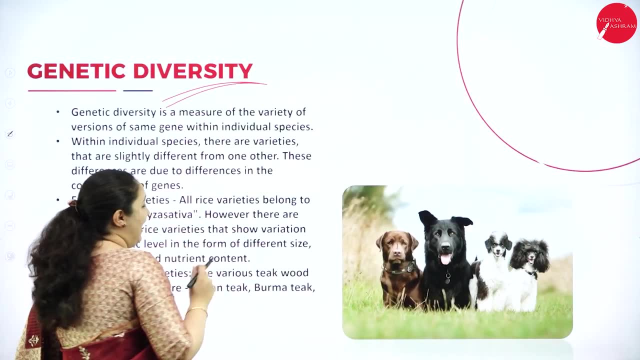 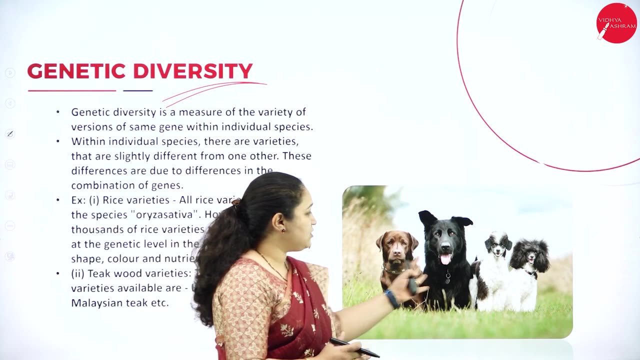 species which we have not yet discovered at all. okay, So that is species diversity. Next we have is the genetic diversity. As I told you, dog is a species, for example, and in dog there are varieties of dog. They all are varying in the genesis. 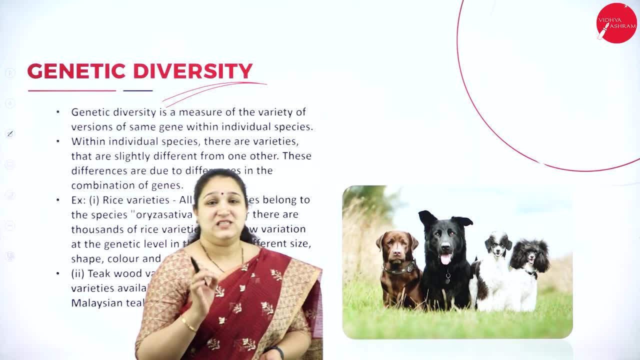 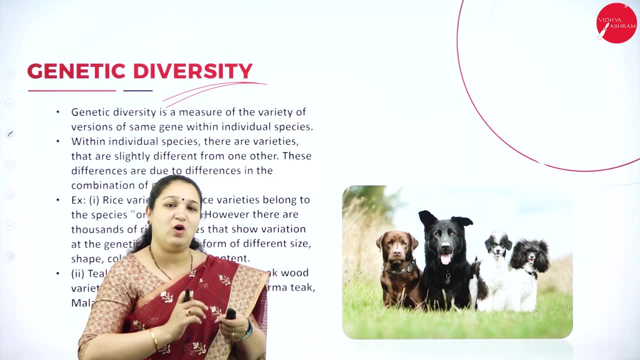 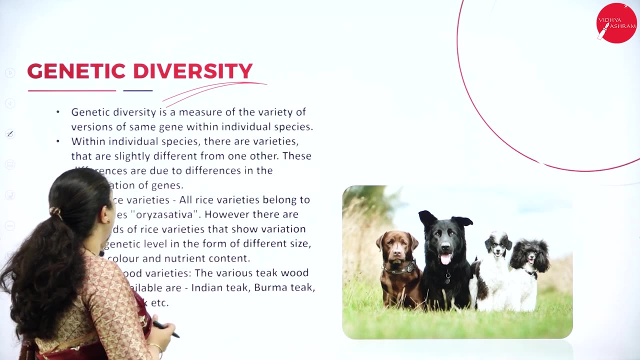 Genetic level and that is called as the genetic diversity. Genetic level means what? In the genes there is a small variation in all of these organism dogs and that is giving rise to different types of dogs, Isn't it So? same way, genetic diversity is a measure of variety of versions of the same. 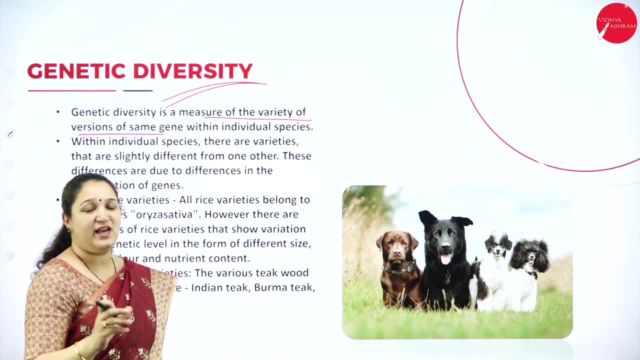 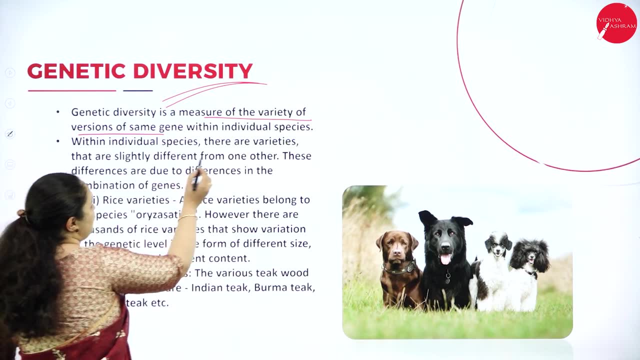 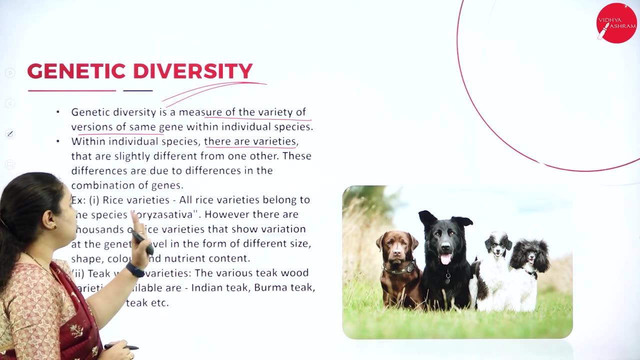 gene. It is a same gene, but there is a small change which is giving rise to different versions of the same, And within individual species there are varieties that are slightly different from one another. The difference are due to the difference in combination of the genes. For example, here we have taken 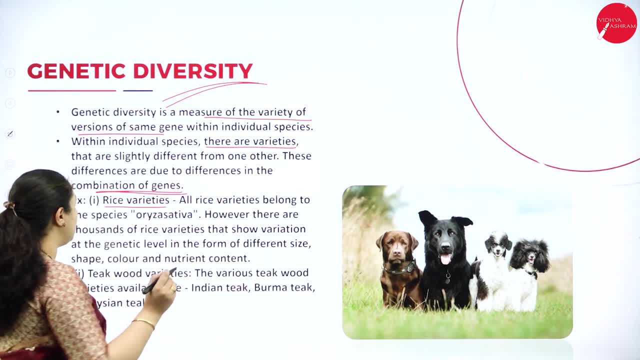 rice variety. Rice variety belongs to the species Oriza sativa, but there are thousands of rice varieties that show variation at the genetic level. Then they are talk about different size, different color and different nutritive value as well. Next, we have even example of Teak wood variety. The Teak wood variety are Indian Teak, Burma Teak and Malaysian Teak. 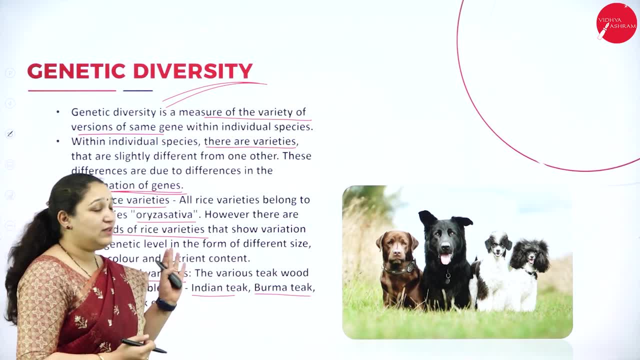 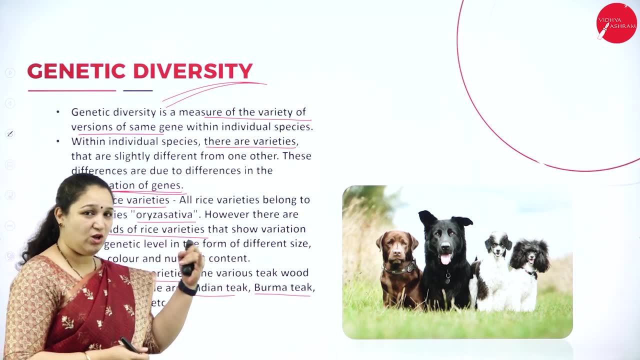 These are some of the Teak wood varieties which we can see. So that is about the genetic diversity. I hope you have understood about the three levels of diversity. One is ecosystem, or ecological diversity- There is species diversity- and the second one is genetic diversity. 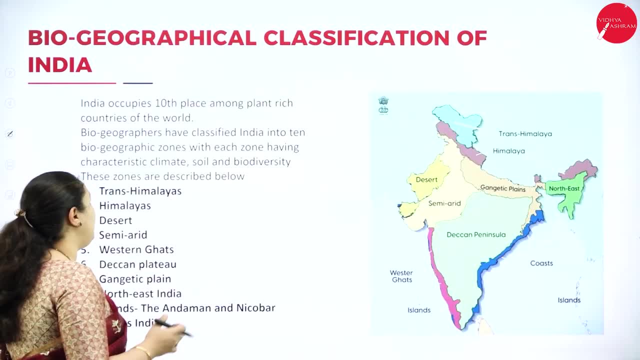 So that's all about the genes. So if you have any question, you can comment in the comment box. Thank you. the genetic diversity next is about the biogeographical classification of india, which is very important question as well. okay, india has got different climate and topography in different 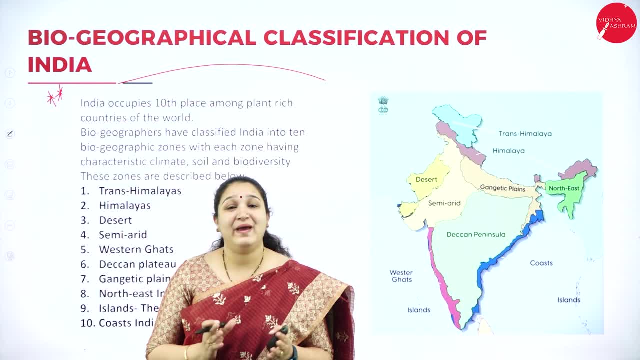 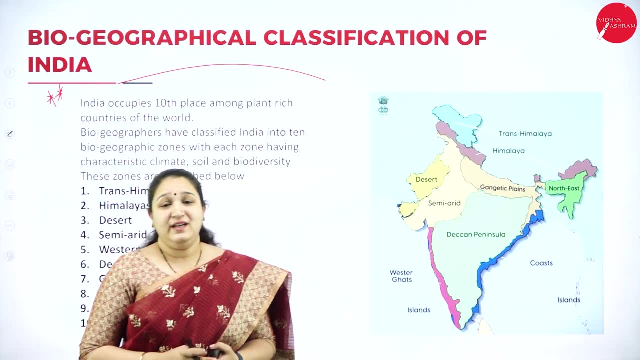 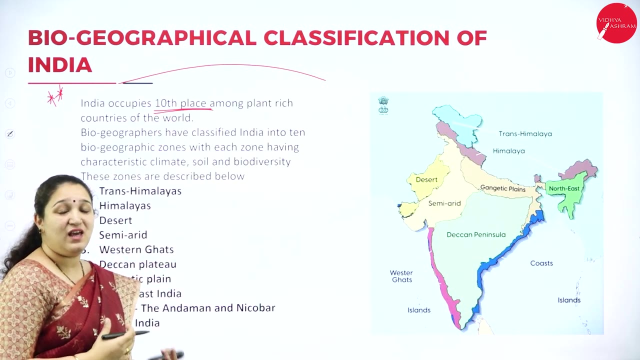 regions, and that is why it is termed as mega diversity country or mega diversity nation. india stands 10th among the plant rich countries in the world. that is the amount of richness which we have when it comes to the different types of plants in india and depending on the climate. 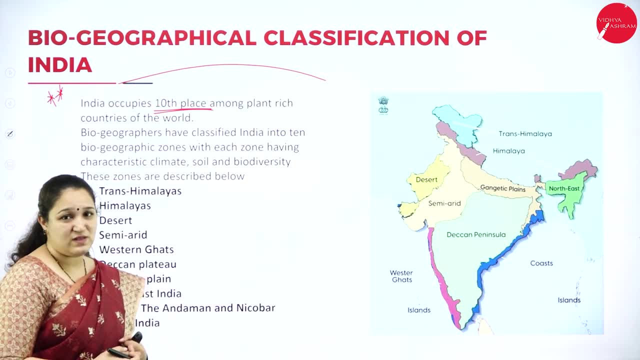 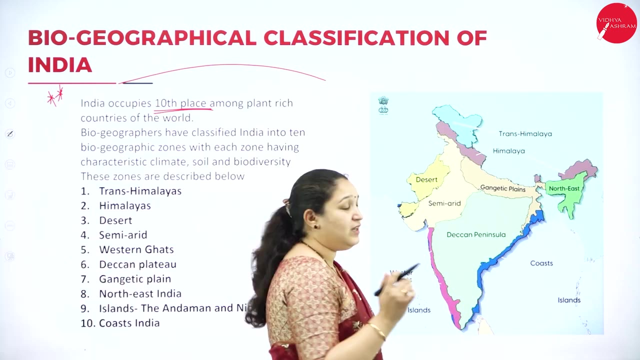 the soil as well as the biodiversity. india has been divided or it can be classified into 10 different zones and that is called as biogeographical zones of india. so there are 10 zones which are there. here you can see. this portion is called as the trans himalayas. here you can see this colored which is there. that is, the himalayas which is. 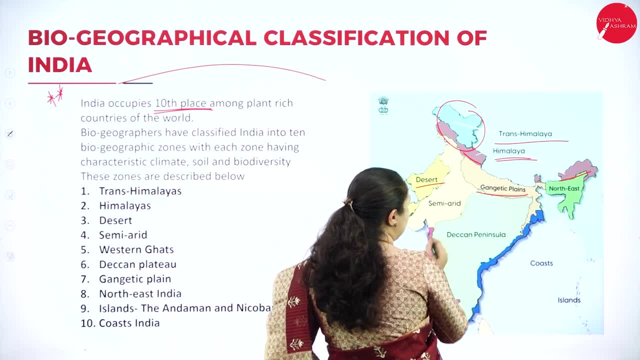 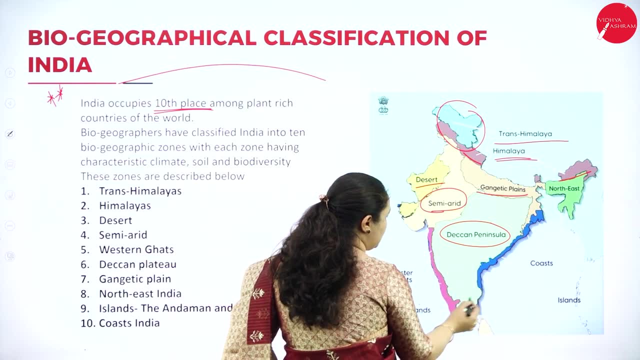 there. then we have the gangetic plain, then we have the deserts. this is called as the semi-arid region. this is deccan peninsula, the coast. you can see there is coastal area. then you have the western ghats, then you have the islands which are there. 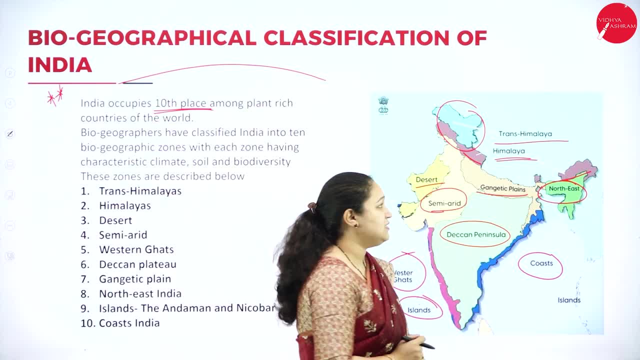 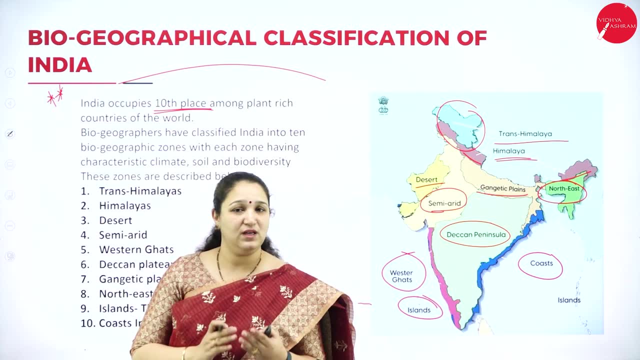 and then you have the deserts which are there, and then you have the deserts which are there, and then you have the north east india, which is there. so these are the 10 different biogeographical zones of india, and we learn each one of them. what is exactly there in that? particular region. okay, so the first one is the trans himalayas. the trans himalayas are the extension to the tibetan plateau, okay, and this region harbors the high altitude cold deserts in india, and this region harbors the high altitude cold deserts in india and this region. 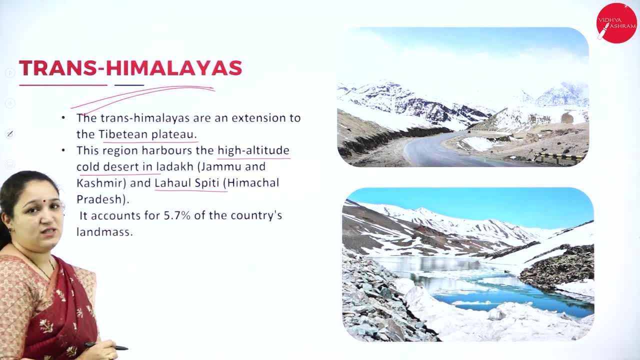 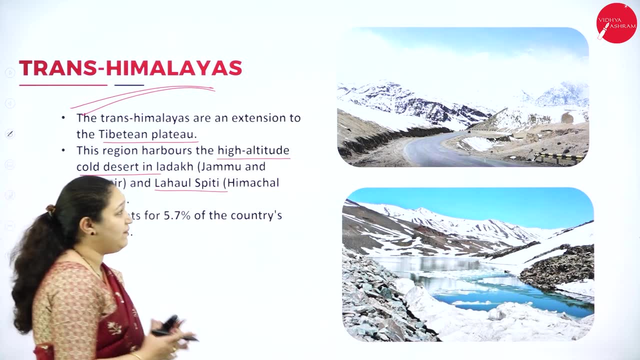 agent has taken over to the south. the south east wind is a main port of lada, as well as lahaul spiti that is present in himachal pradesh. it has got cold. deserts mean it's very, very cold. you can see it is all having the mountains with lot of ice in them. that's why they are also called. 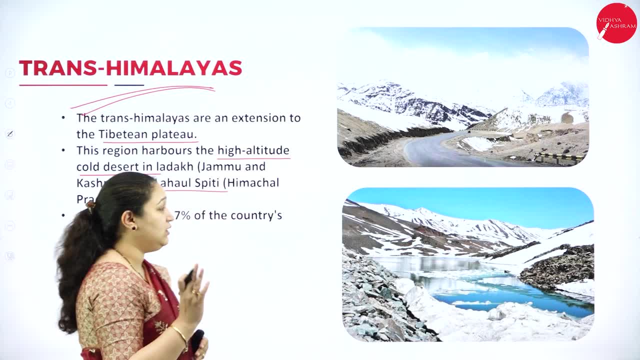 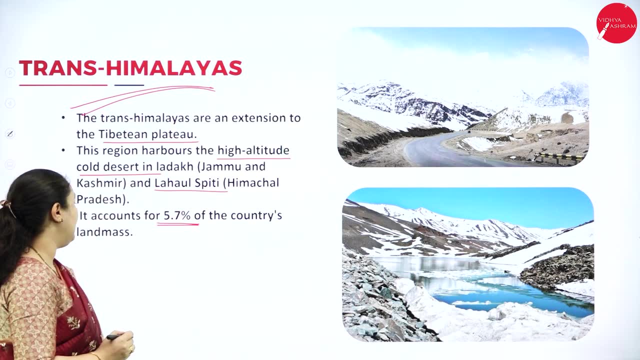 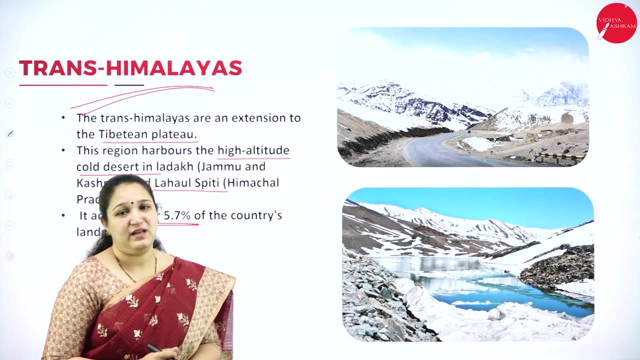 as cold deserts of ladakh, okay, and it accounts for 5.7 percent of the country's land mass. how much, 5.7 percent of the country's land mass? okay, and now we come to the second one. this is the of the land is there in trans-Himalayan regions. 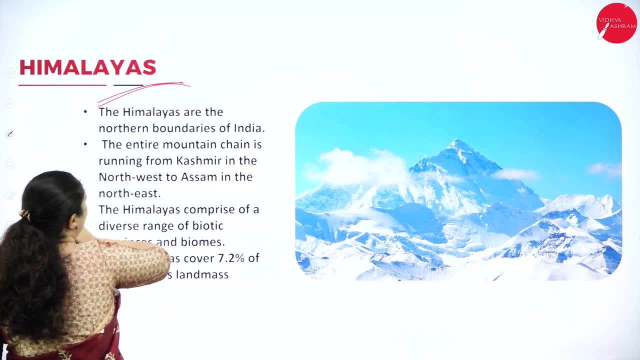 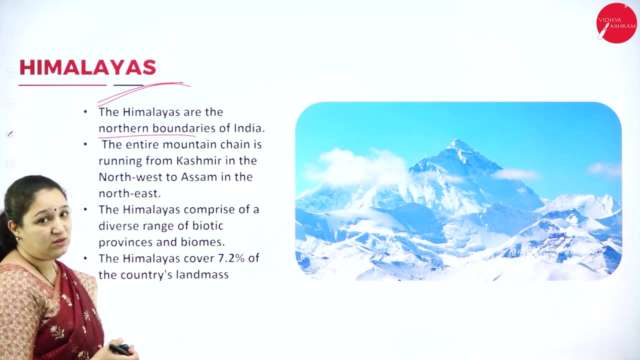 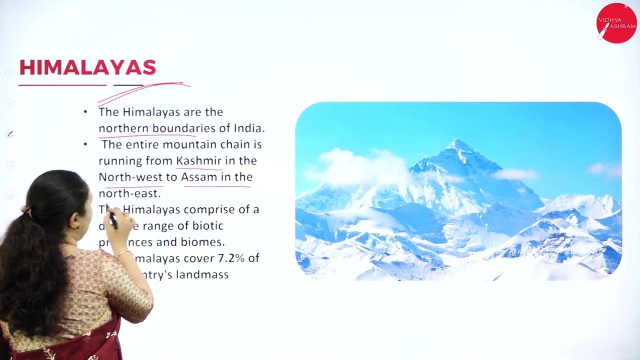 Next we have the Himalayas. The Himalayas are the northern boundaries of India, isn't it? That comes in the boundary region, so they are called as the northern boundaries of India. The entire mountain chain is running from Kashmir in the northwest to Assam in the northeast. 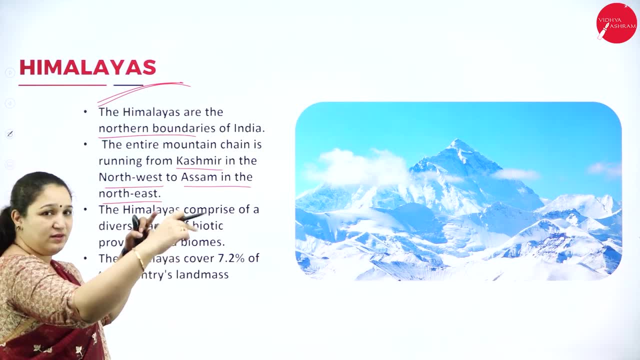 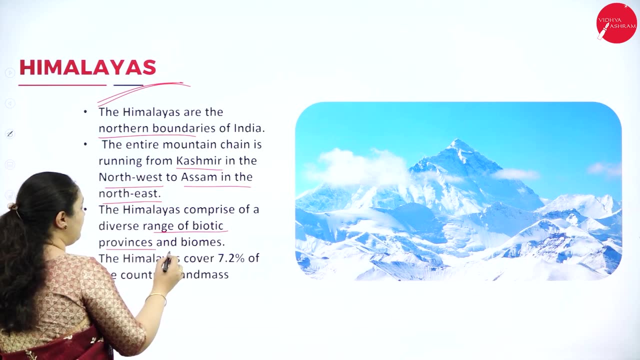 So from the northwest to the northeast they are running and they are forming the boundary of India. The Himalayas comprise of diverse range of biotic province as well as the biomes, That is, they have very rich, different kinds of living beings in them. 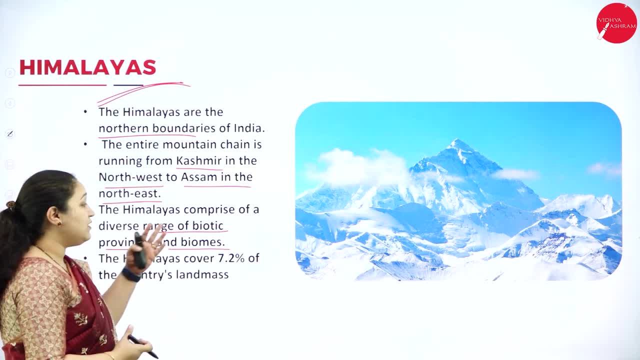 That's why we call it as it's very rich in different, diverse range of biotic provinces, as well as the biomes. Biomes is a region in which all the living organisms are there and that is very rich or different type. it is present okay. 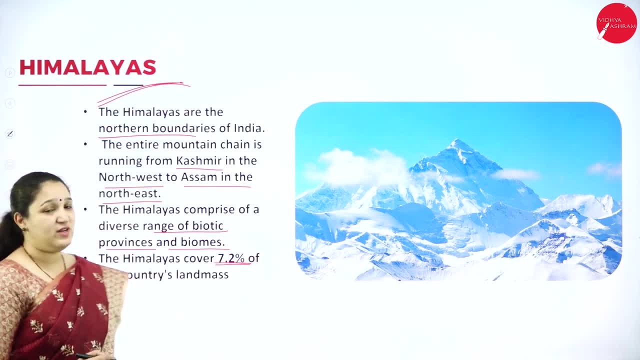 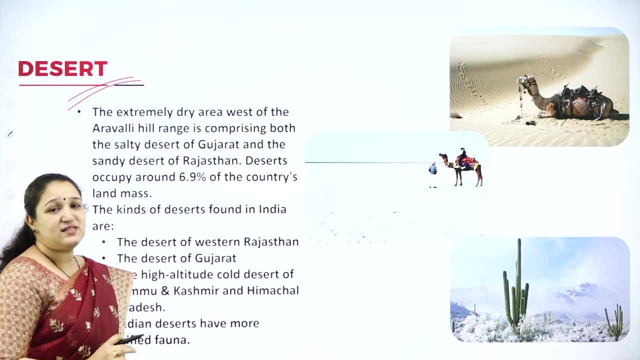 And Himalayas cover up to 20,000 hectares, So 7.2% of the country's landmass. Next we have the deserts. What are deserts? It is extremely dry areas of west of the Aravalli hill range. 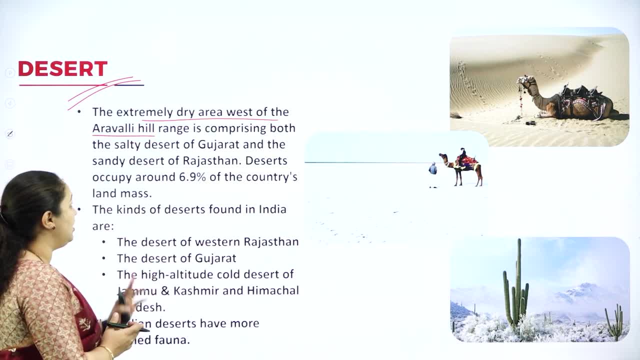 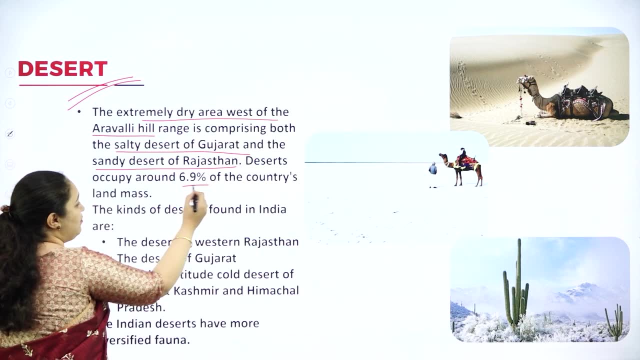 It is present in the west of the Aravalli hill range and it comprises both salty deserts of Gujarat and the sandy deserts of Rajasthan. So it is taking up to 6.9% of country's landmass And there are three kinds of deserts which we can tell. 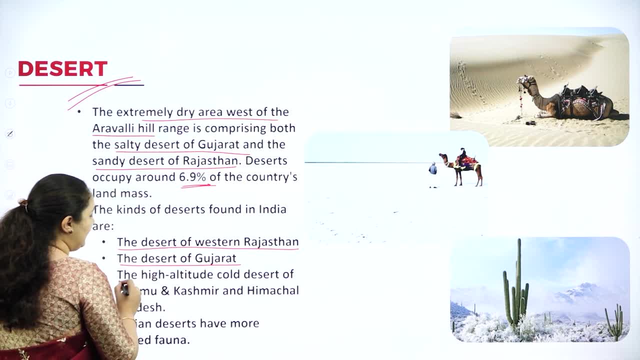 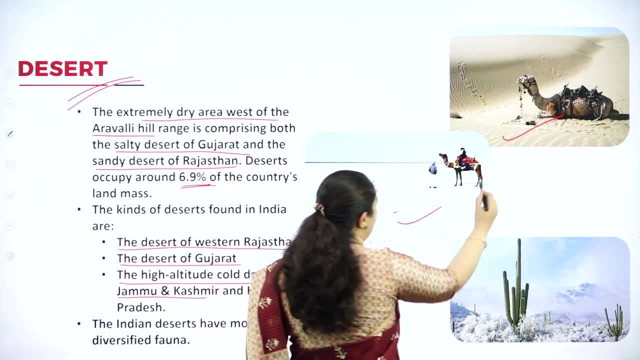 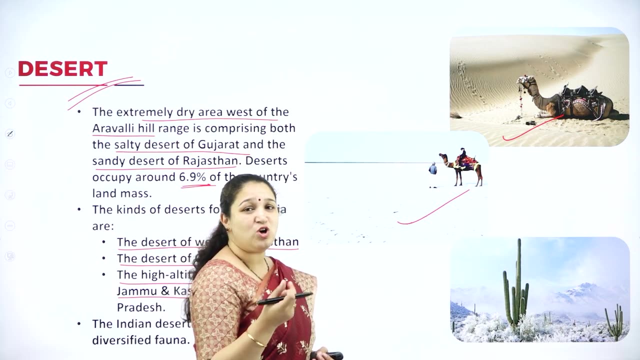 The deserts of western Rajasthan, the deserts of Gujarat and the high altitude, cold deserts of Jammu and Kashmir. You can see here. this is the deserts of Rajasthan. This is the deserts of Gujarat. We call it as salty deserts of Gujarat. where you can see there is. it looks like salt, which 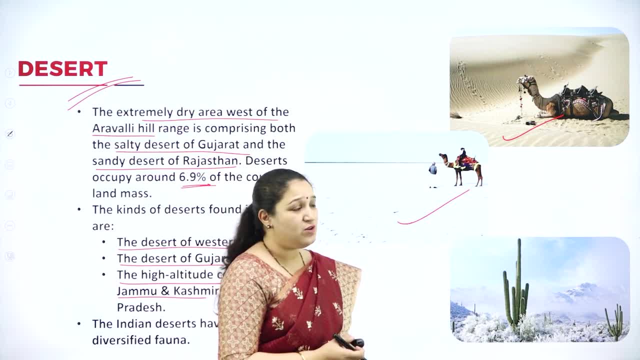 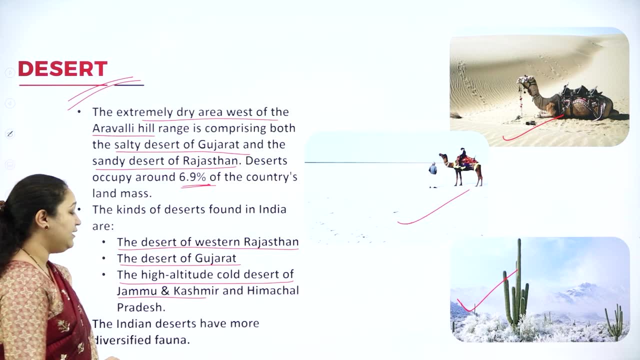 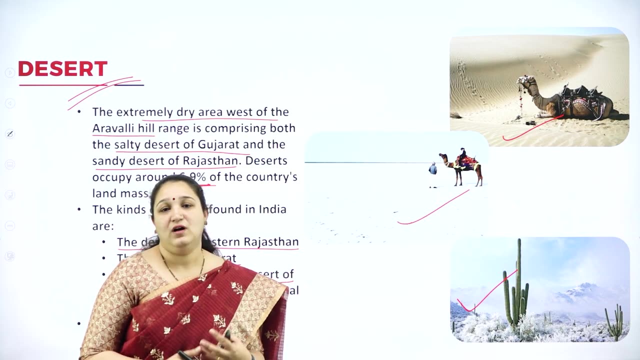 is there, It is white color, okay, And that is sandy deserts of Rajasthan and the cold deserts of Jammu and Kashmir and Himachal Pradesh is present here. The Indian deserts have more diversified fauna in them, So deserts, we know they have a different kind of ecosystem altogether. 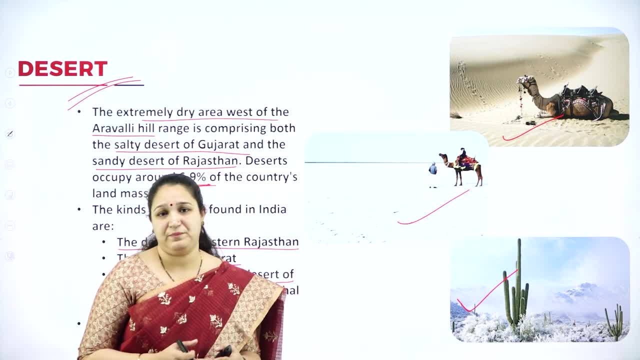 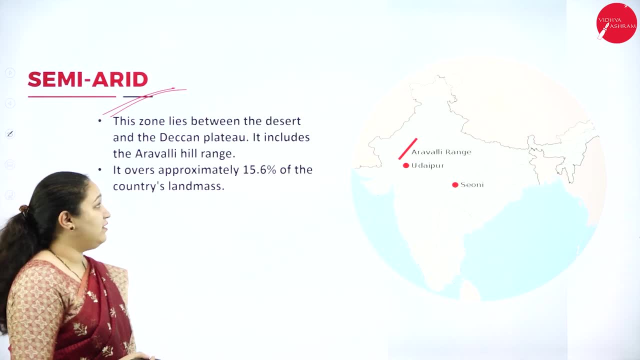 They have different kinds of plants as well as animals living in them, isn't it? Next, we have about the semi-arid region. The semi-arid region- you can see, it is there over here, And it has the arid deserts. 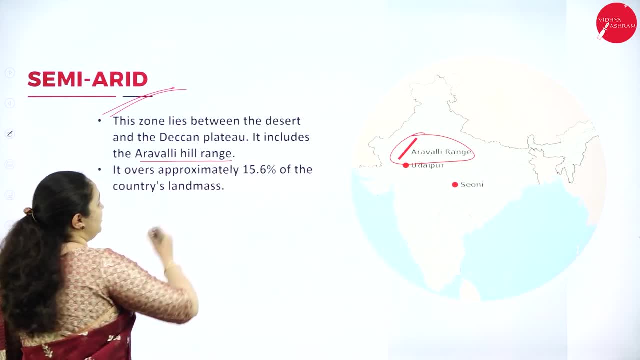 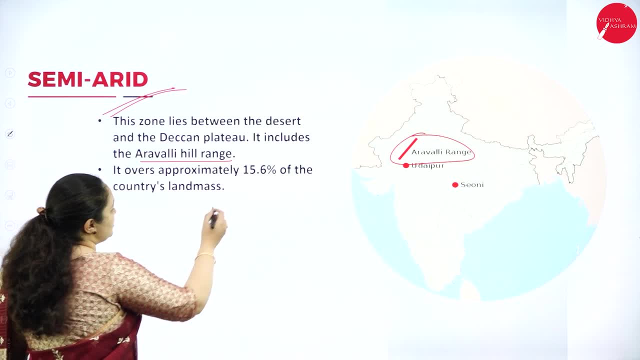 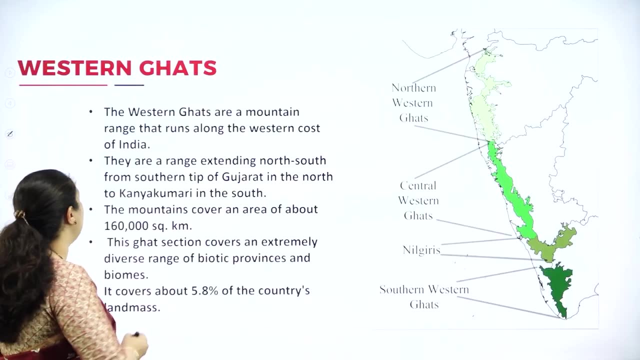 That hilly region is called as the Aravali Hill range And it covers approximately 15.6% of the country's land mass. okay, Next region is called as the Western Ghats, one of the hotspots of India, we can tell. 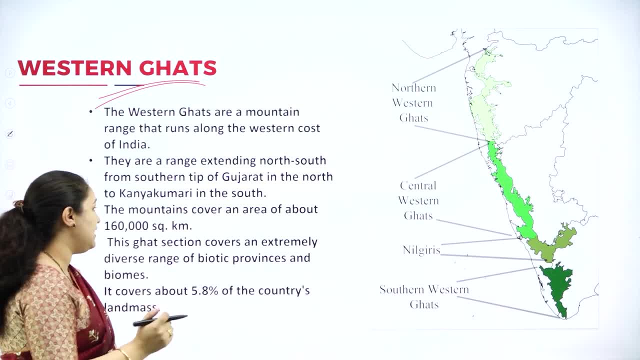 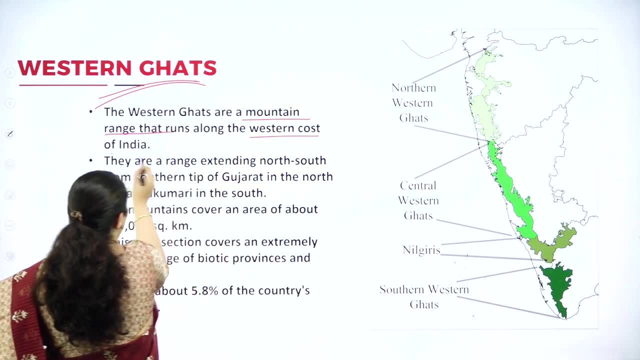 That is why hotspots I shall explain in the next class. but western ghats are the mountain range that runs in the eastern region And in the western region. this is called the mountain range range that runs along the western coast of India. the western coast of India. what is it? this is the 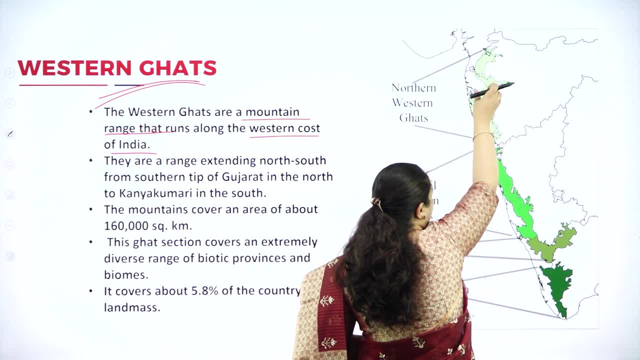 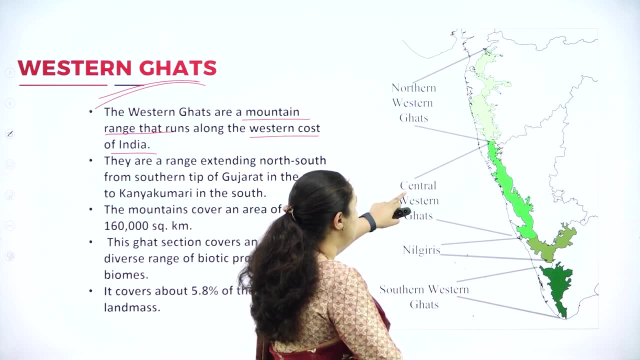 coastal region. just next to that, you can see, there is, you know, complete hilly region which is there which is called as the western guards. you can see, this is called as a northern western guard, central western guard. then we have the Nilgiris and then we have the southern western guards. okay, 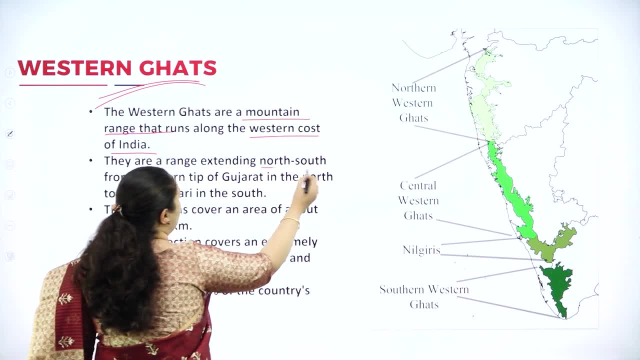 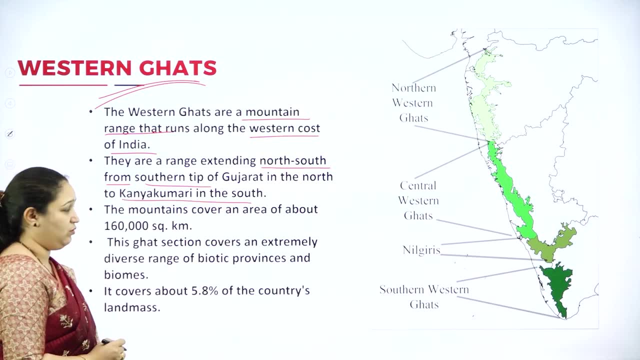 they are range extending from north south, from southern tip of Gujarat in the north to Kanyakumari in the south, okay, and the mountain covers the area about 160,000 square kilometers. that is a very huge area which it covers and this guard section covers extremely diverse range of biotic. 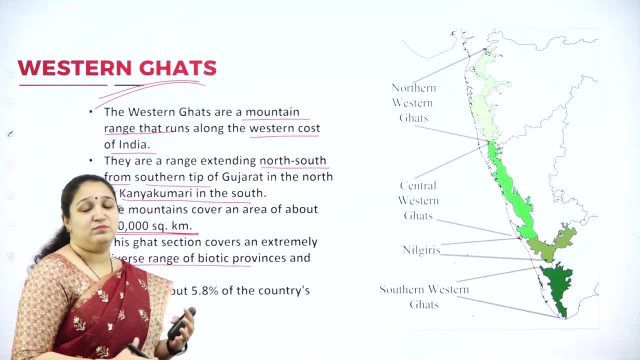 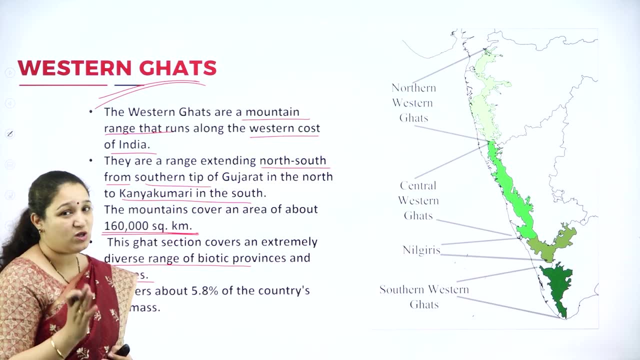 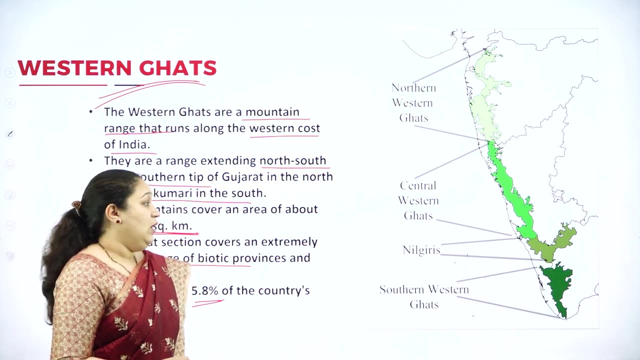 province and biomes, that is, they have a different, you know, types of plants and animals which are living here in the western guards, and that's the reason we call it as the hot spot of India as well. it covers about 5.8 percent of countries landmass. more about western guards and about 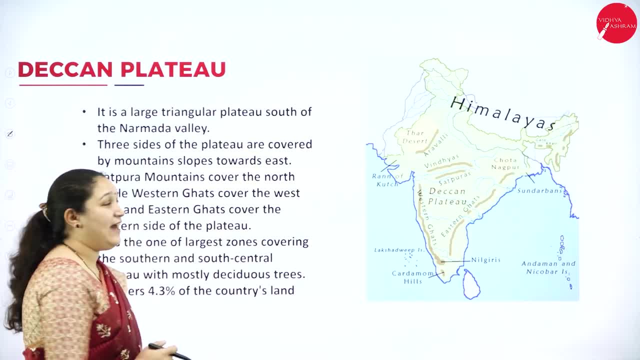 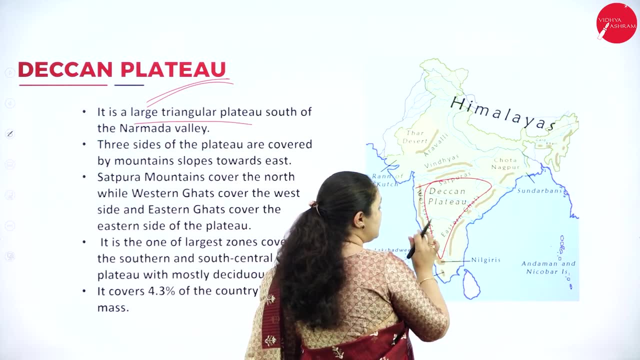 the species living there. we learn in the next class. okay, next we have the Deccan plateau. Deccan plateau is a large triangular plateau which you can see like this: it is covered with all the three sides, with the mountains you can see here. here we have the western guards in the west and the 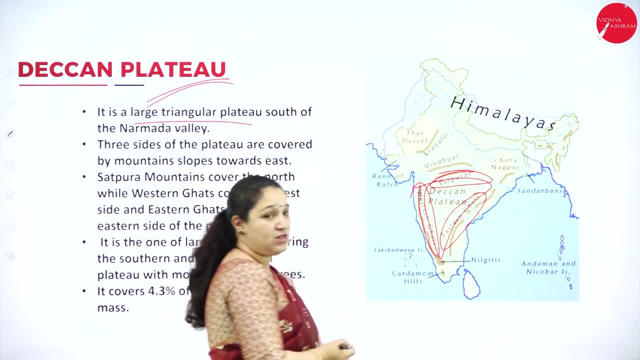 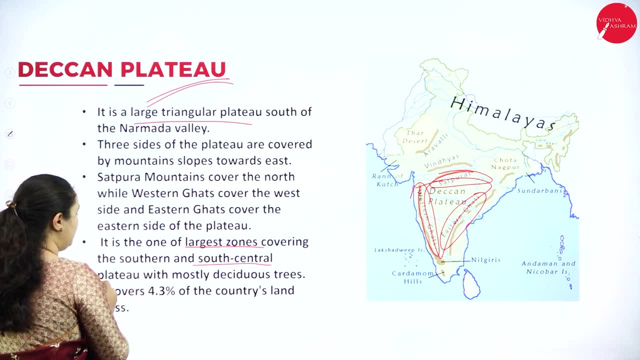 eastern guards in the east and Satpuras in the north side of the Deccan plateau. it is one of the largest zones covering the southern and the southern central plateau, with mostly deciduous trees. here they have deciduous trees. deciduous trees are those trees which shed their leaves. 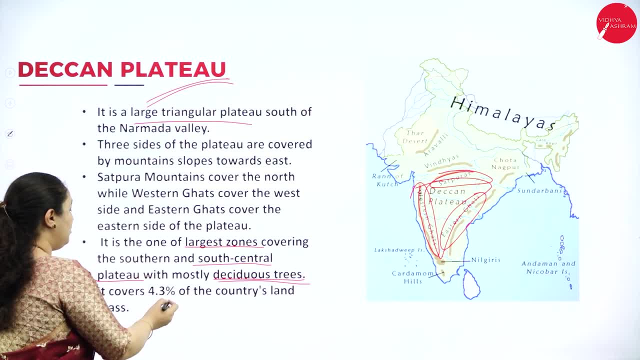 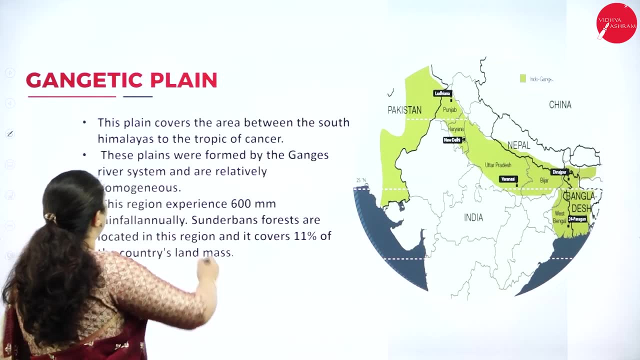 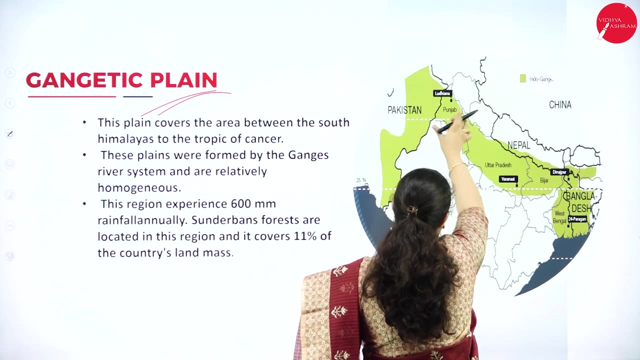 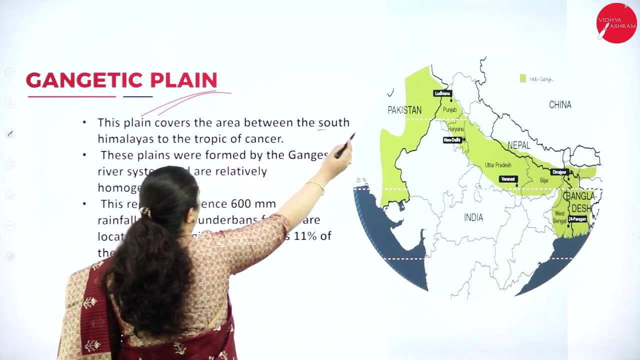 during the winter- okay, it covers about 4.3 percent of countries landmass- okay. next we have the Gangetic plane that comes just below the Himalaya region. you can see this is the Gangetic plane, which is there. okay, this plane covers the area between the south Himalayas to the tropic of. 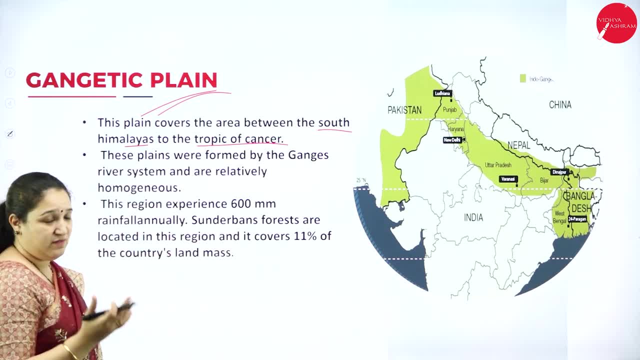 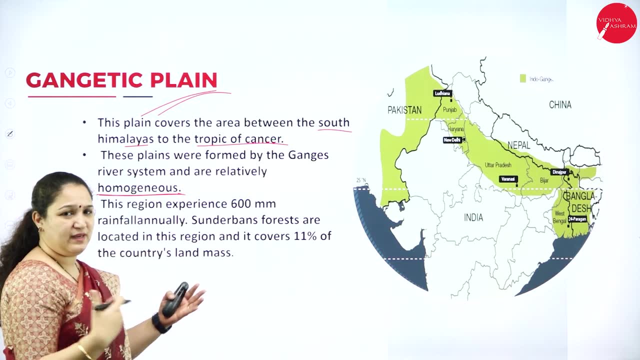 cancer. these planes were formed by Ganges. that is the river Ganga, and it is relatively homogeneous. okay, that is almost. it's all of the same type. that area is almost of the same type and this region experiences 60 millimeter of rainfall annually. Sundarban's forests are located in this. 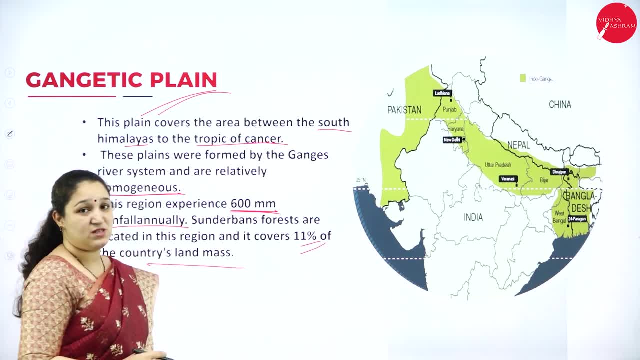 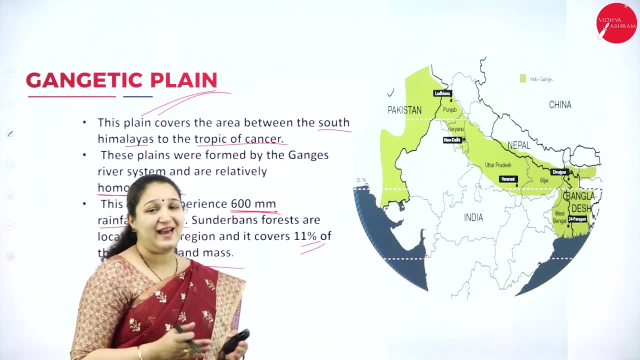 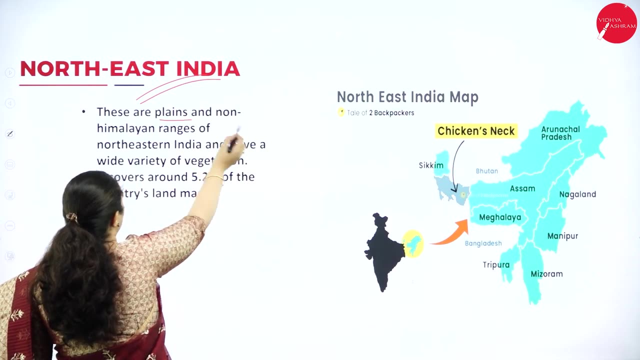 region. it covers about the 11 percent of the country's landmass. Sundarban is the forest area which is there in this, you know, Gangetic plane region. next we have the northeast India. the northeast India- there are planes- and the non-Himalayan region of the northeast. you can see. 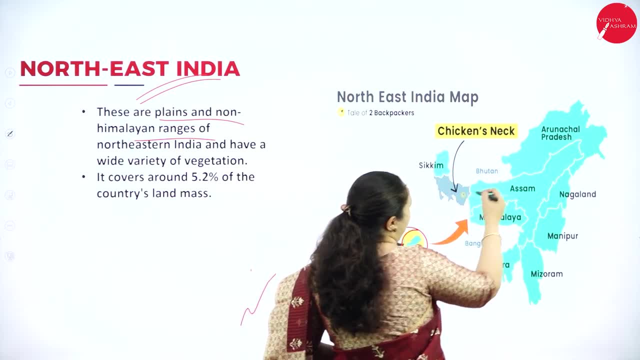 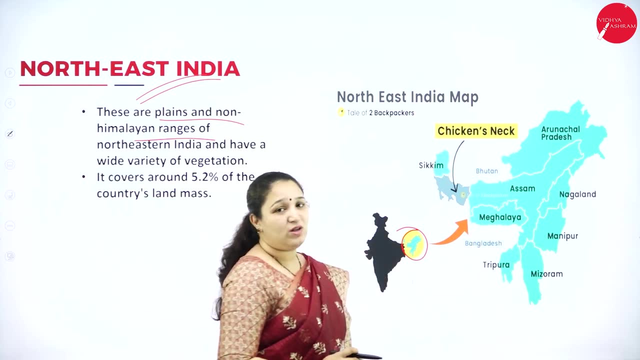 this is northeast India, so you can see. this is the north east India, so you can see the north east India. so here you can see, from Sikkim, here, Arunachal Pradesh, you have Nagaland, Manipur, Mizoram, you know, Meghalaya, Assam, all of this comes under northeast India. they have a wide variety of you know. 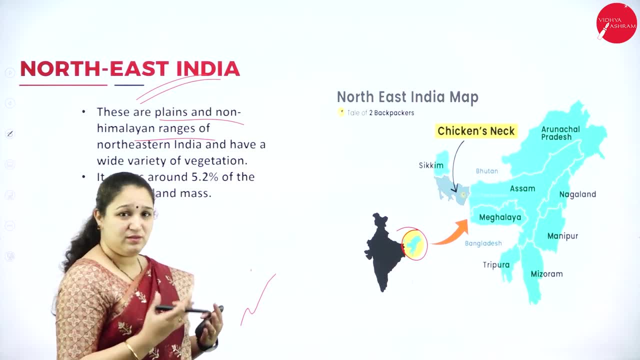 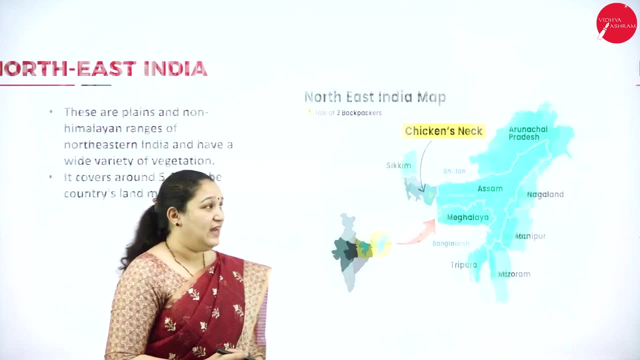 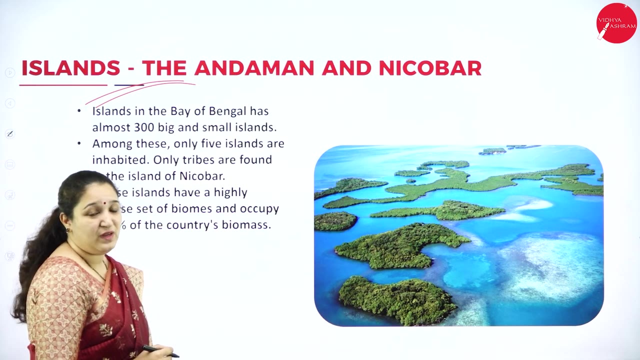 vegetation and it rains really a lot in places like Assam as well, and it covers about 5.2 percent of the country's landmass. okay, next we have the islands, the Andaman and Nicollet- okay, these are the islands. we can tell the tribes really are still existing here. there are so many. islands which are not even having human habitation, in Andaman and Nicobar. so islands of Bay of Bengal have almost 300 big and small islands. there are so many islands, out of which only five islands are inhabited. only tribes are found in islands of Nicobar, okay. and these islands have highly diverse set of biomes and occupy 0.03 percent of country's biomass, but they have a very vary, wide variety of endemic species in them and they are very, very rich in their biodiversity. okay, even if the landmass is really very less, there are so many. 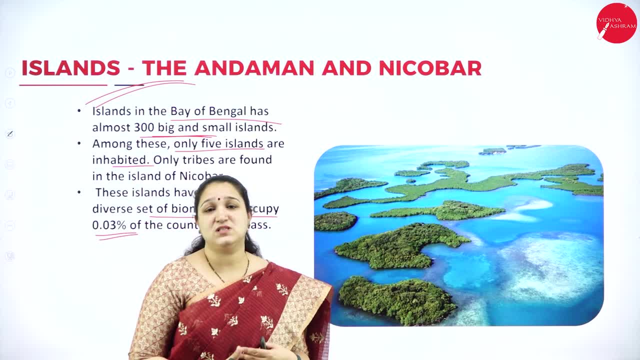 islands which are not, it you know, having any humans habitation at all, as well as they are not discovered many islands. they are not yet 친구 Russia at all, as well as they are not it discovered. so many islands, they are only tribes of Right you. 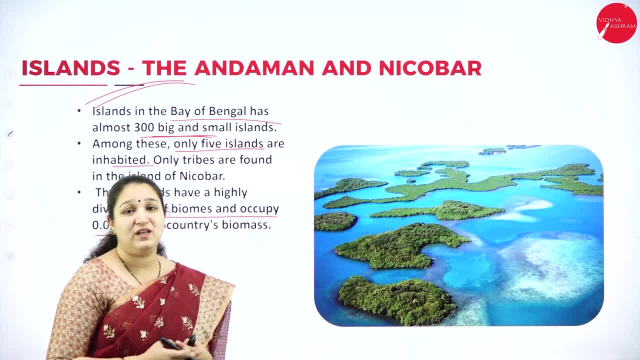 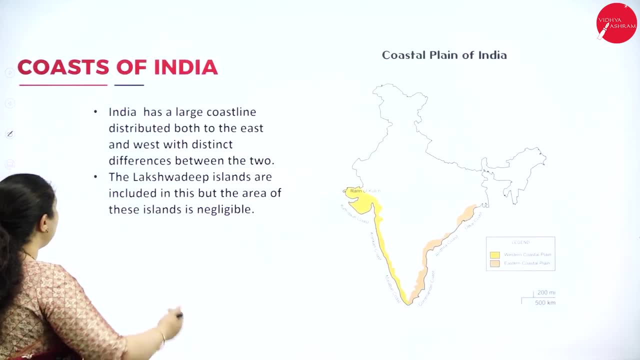 who live there. ok, so humans are not intervening there and the biodiversity is really, really rich in islands of nicobar, ok. next we have the coasts of india. india has a large coastline distributed on both the sides. we know we have two seas on both the sides of india and that's. 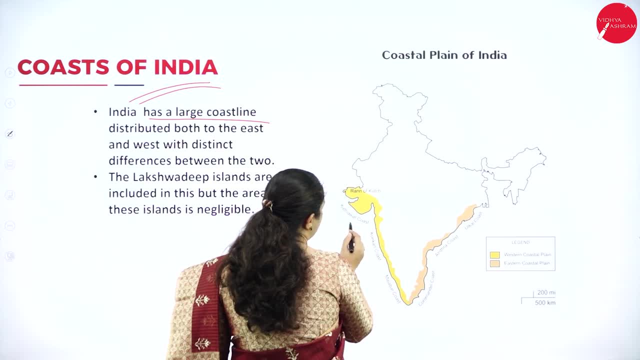 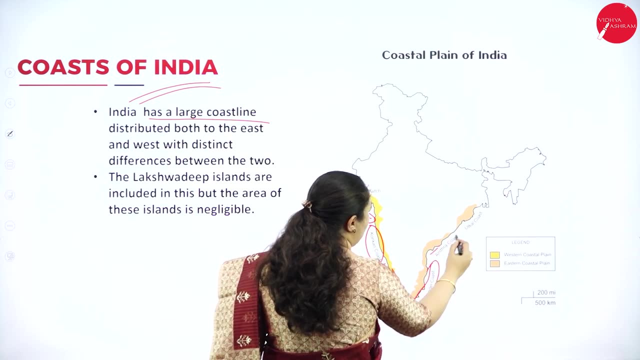 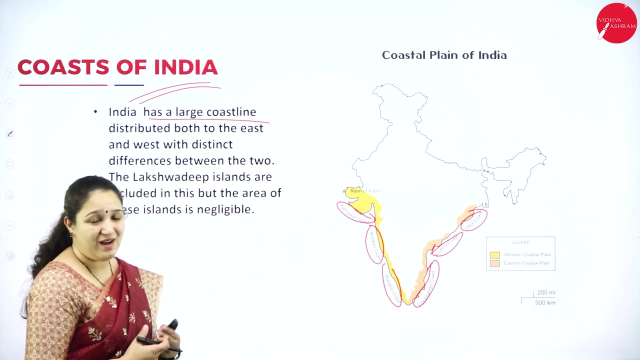 why the coastal region is a lot, then you you can see here kathiyavar coast, konkant coast, malabar coast, then you have koramandal coast, andhra coast and also utkal coast, which is there. so on both the sides you have seas and there is a large coastal area which we have. 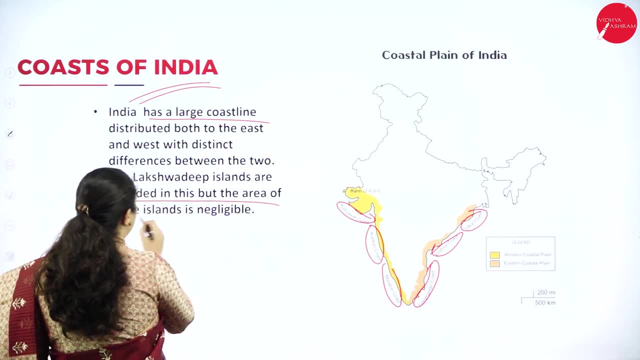 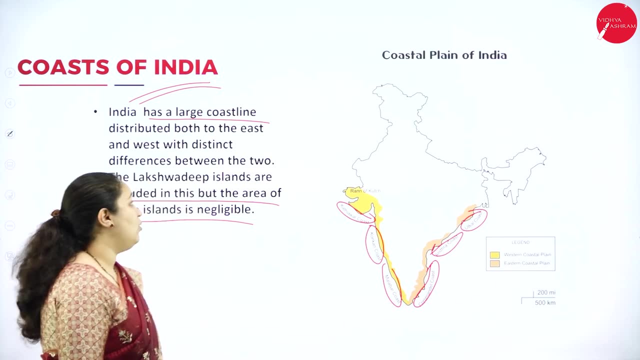 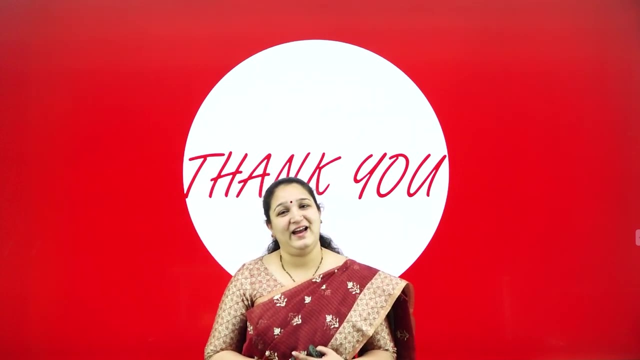 the lakshadip islands are also included in this, but the area of these islands are really negligible because they are very, very small areas. ok, so that's about the coasts of india. i hope you have understood about the biogeographical classification of india and 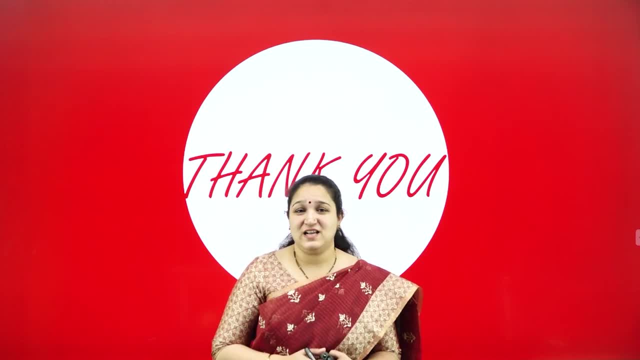 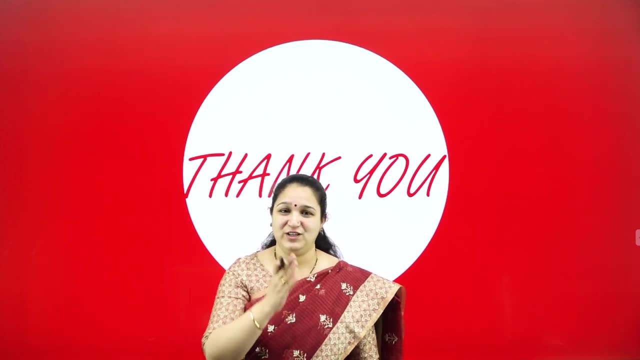 also about the biodiversity. next class we'll be learning about the other species of india. thank you, my dear children. stay tuned for more updates.